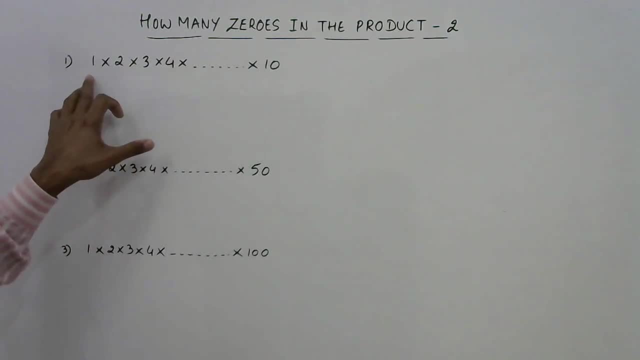 So if we have a series like this, like the numbers starting from 1 and ending at 10, and all numbers are multiplied together, See, we cannot assume that we can find the product and then find the number of zeros which will come at the end of the product, because that is going to consume a lot of. 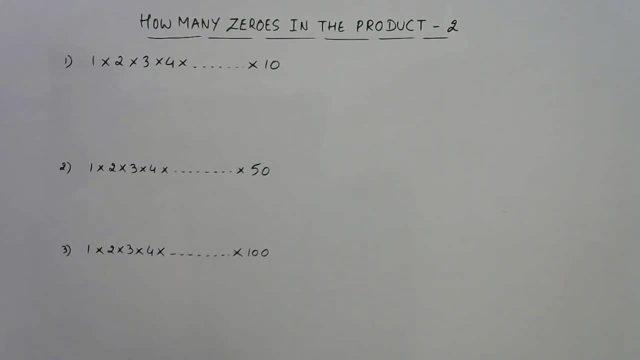 time. So we need a method through which we can find out the number of zeros easily. Secondly, the method which I told you like to factorize each and every term of the given product. that will also be very tedious here, because in the first case it is only 10 numbers, but in the second 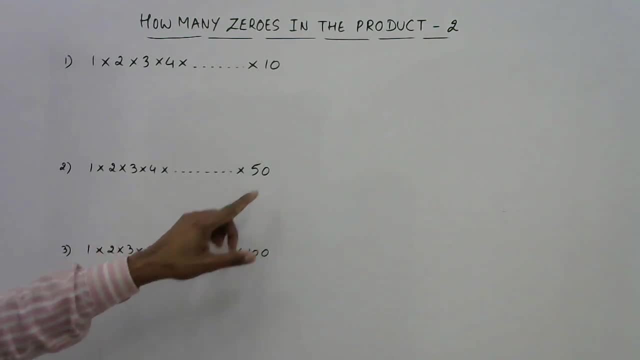 case. you see, I have written the product up to 50 and here I have written the product up to 100. So it is impossible to make factors of all the numbers and sort out the number of 2s and number of 5s. So to find the number of 2s and number of 5s, 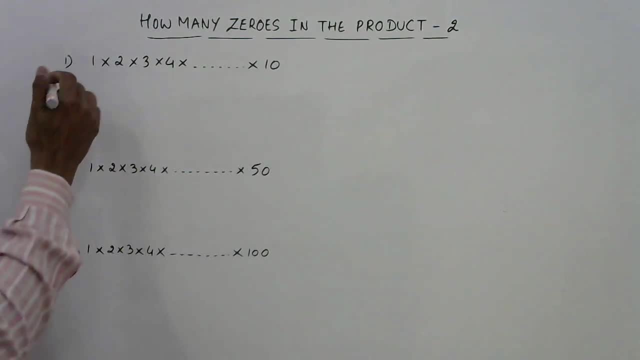 I have a method for you: See the number of 2s, How you can find the number of 2s? Just see the last number here. Last number is 10 and, mind you, no number should be missing and the series should start with 1.. So last number is 10 and we want to find the number of 2s. So divide it by 2. 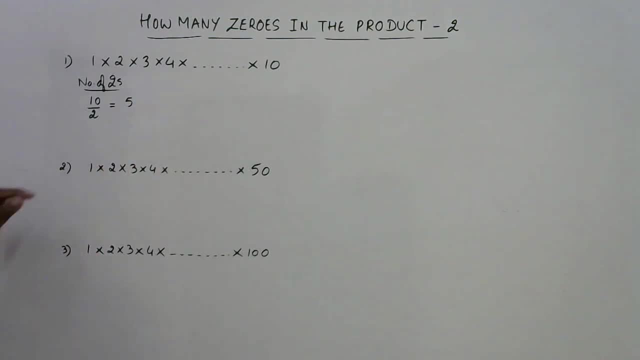 you get 5.. Now 5 is greater than this divisor 2.. So we can again divide 5 by the same divisor 2.. Now you get 2 as the quotient and 1 as the remainder. Just forget the remainder. 5 divided by 2 is 2 point. 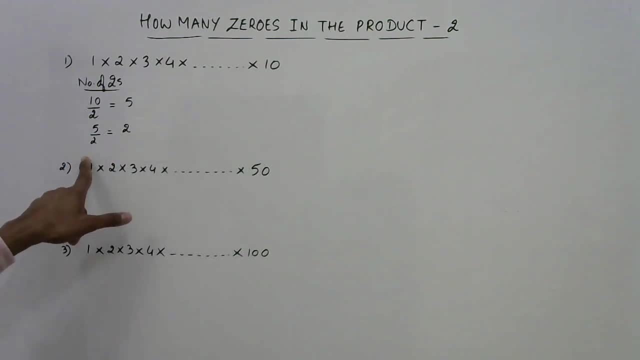 something. so I will write only 2.. Now 2 and 2, they are equal, so we can divide again. So in the final step, we will have one more step like this, in which we will be dividing the number of 2s. We will be dividing 2 by 2.. You get 1, and now 1 is less than 2.. So this is what we want. We keep on. 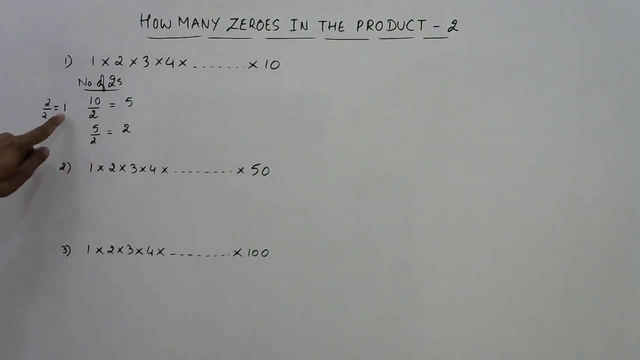 dividing. when we get a number quotient which is less than the divisor, then we stop And now just count 5, 6,, 7,, 8.. So there are 8- 2s in this product. You don't need to factorize each and every term. 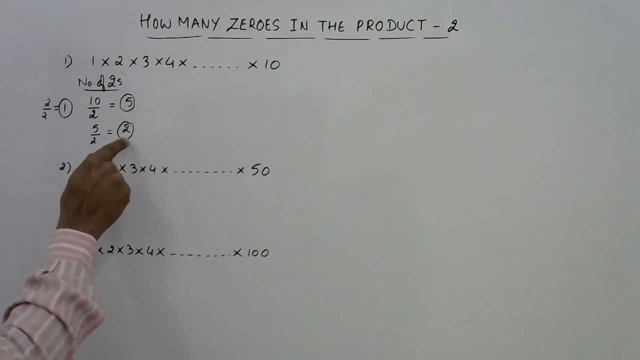 here. Just follow this. Follow this procedure and you will find the number of 2s. Similarly number of 5s: See last number is 10 and now the divisor becomes 5.. This gives you 2.. Now 2 is less than 5.. So there are only 2 5s in. 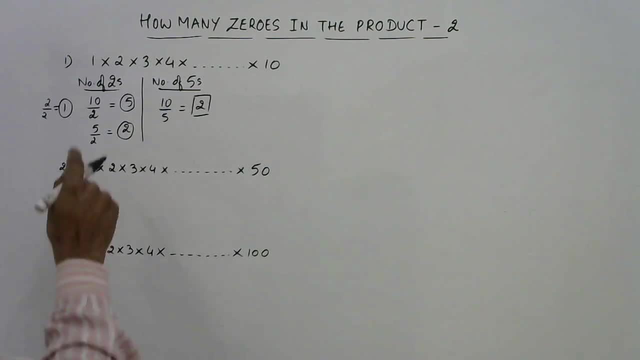 this product. How many 2s, 8, 2s, How many 5s? 2, 5s. So your answer will be minimum of number of 2s and number of 5s, 8 and 2, which is equal to 2.. So your answer is 2: 0s in the product. 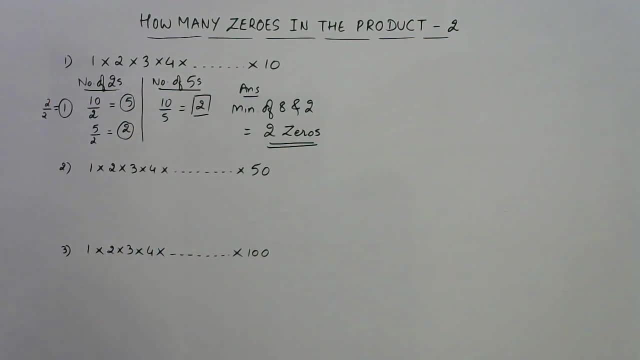 So a very, very important concept again for finding the number of 0s in a given product like this: Now, if you know the method, let us apply the trick here. Number of 2s: See, this is 50. So 50 divided by 2 is 25.. Now 25 is much larger than 2.. So we will divide again. 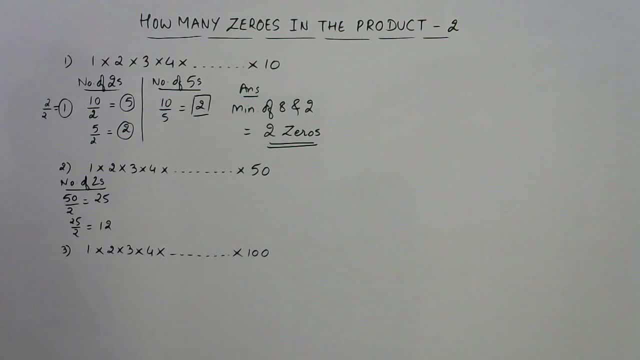 25 divided by 2 is 12.. 12 is again larger. So 12 divided by 2 is 6.. 6 divided by 2 is 3.. And 3 divided by 2 is 1. As a remainder, just forget the remainder Now. number of 5s: 50 divided by 5 is 10 and 10 divided by 5 is 2.. See the answer. 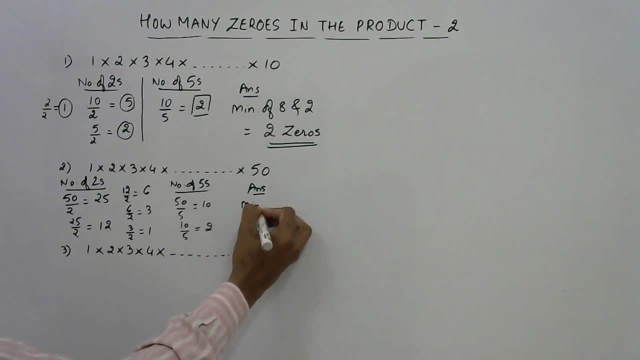 Number of 0s minimum of see 25,, 37 and 47.. So there will be 47 2s and 12 5s in this product. So now the answer is 5.. So the answer will be 7.. So 3 divided by 2 is 16.. How many? 1s, 8, 5s? The answer is 3. prey and 12 gold coins. Now this number has algae in it. Now this number must be doubled in the product So자 2s. So it isも estim некоторgestellt. 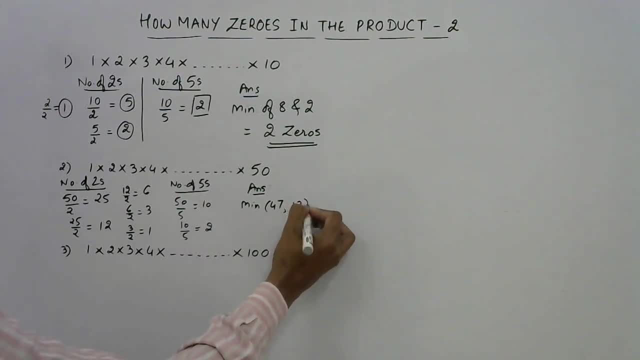 Number of 0 с is allowing to be multiplied by 2 s and therefore, compared to 1 c of zinc, you can skip this number and divide into 10 and 2s, 12, 5s in this product, thereby giving you the answer: 12,, 12, 0s. Friends, once you know this, 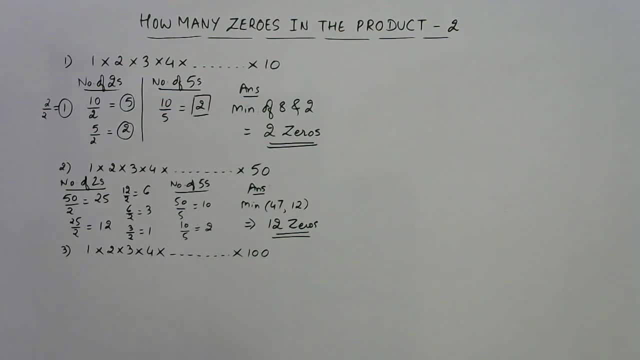 method. now you can reduce the complexity further How I will tell you. Just observe that the number of 2s will always be greater than number of 5s. Here also, number of 2s is much larger than number of 5s, So we need to take the minimum of the 2.. So just find the number. 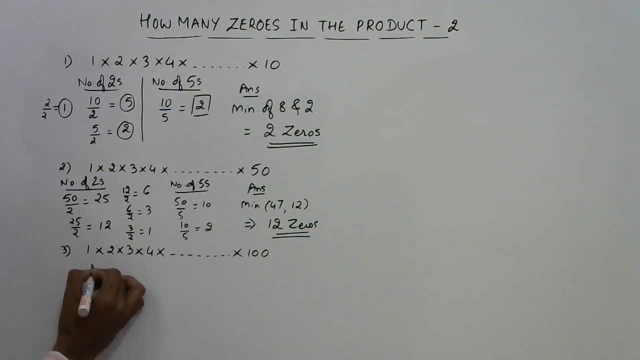 of 5s. So let us solve this using this method. Number of 5s. See, there are total 100 numbers. So 100 divided by 5 gives you 20.. 20 divided by 5 gives you 4.. Now, 4 is less than 5.. So 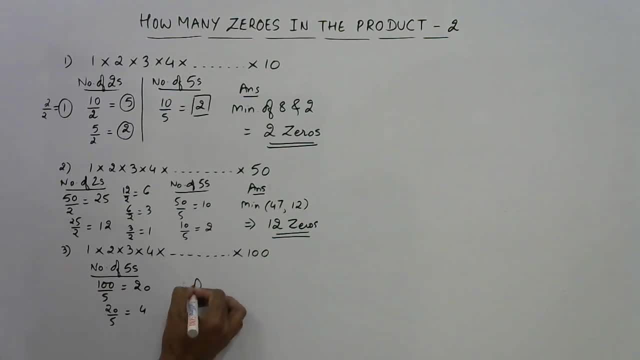 total number of 5s are 24.. Therefore, your answer for the question will be 24: 0s. So, friends, now I have reduced the complexity further and instead of finding 2s, you can find only the number of 5s and get to your answer very, very quickly.